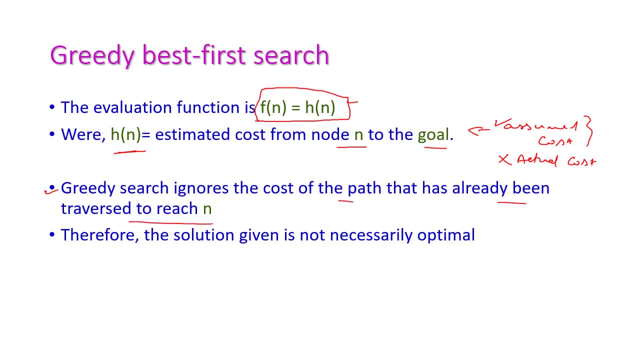 path that has already been traversed to reach the node. okay, already visited nodes will not be considered for traversing further and therefore the solution is not necessarily optimal. that is the greedy best. first searching algorithm is not an optimal algorithm, and let us see one example. 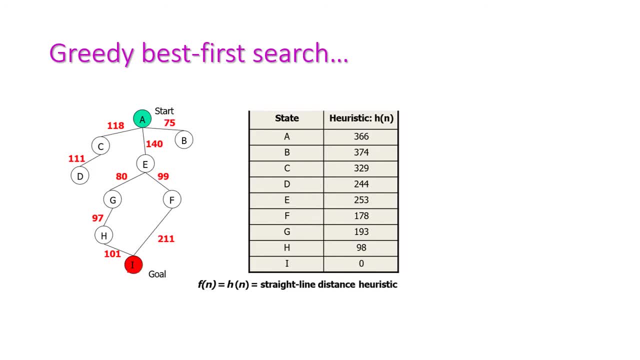 for this greedy best first search. and this is the graph, problem graph. this is the problem graph and this is the heuristic table. both will be given in the problem itself, right, and here we are having this starting node and this is our goal. okay, and by using how this greedy best first search. 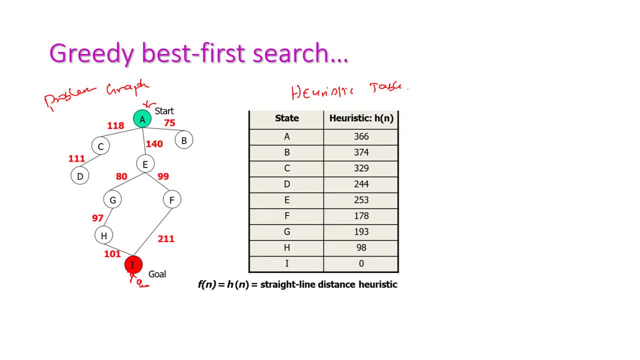 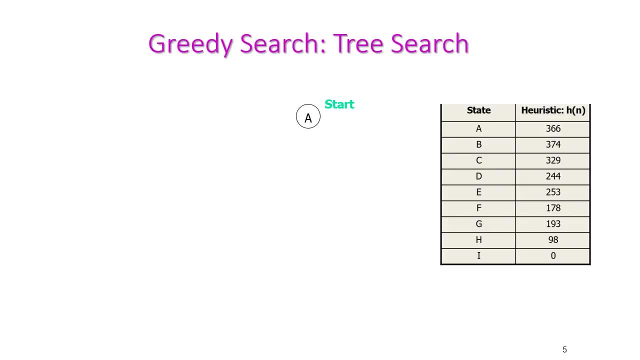 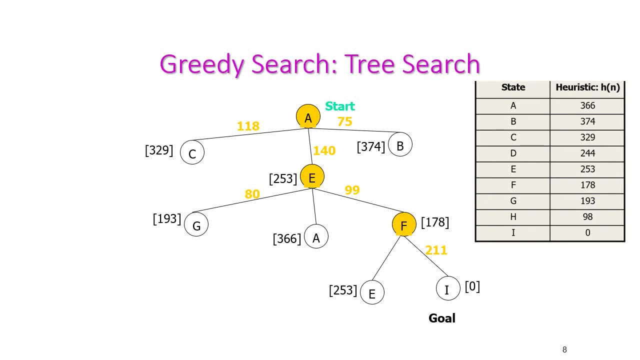 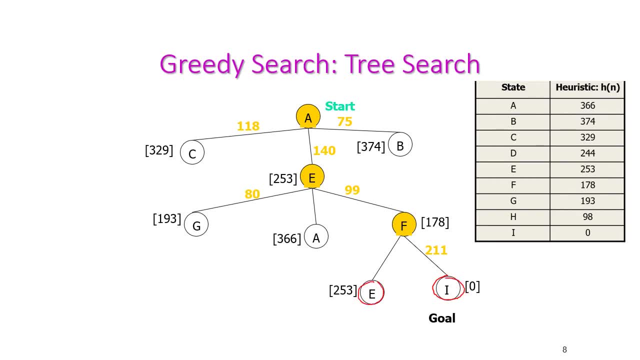 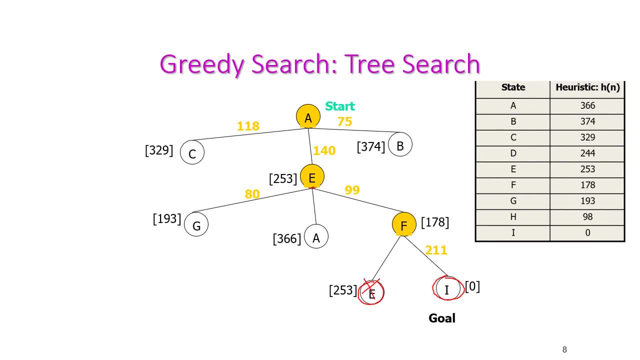 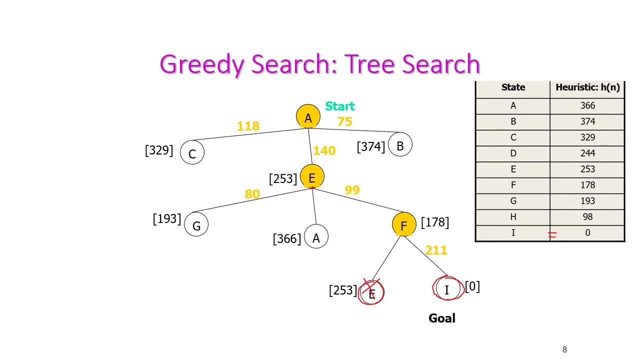 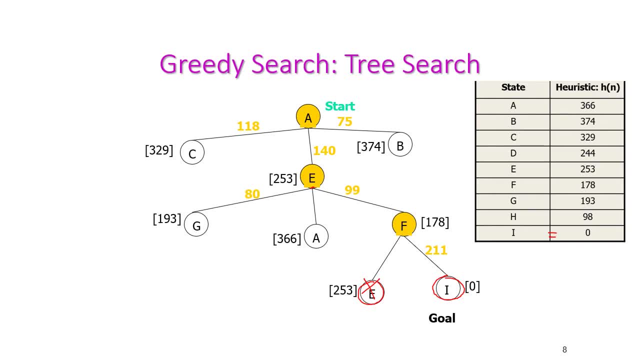 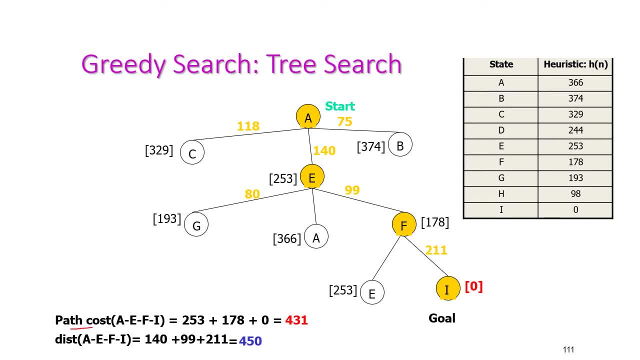 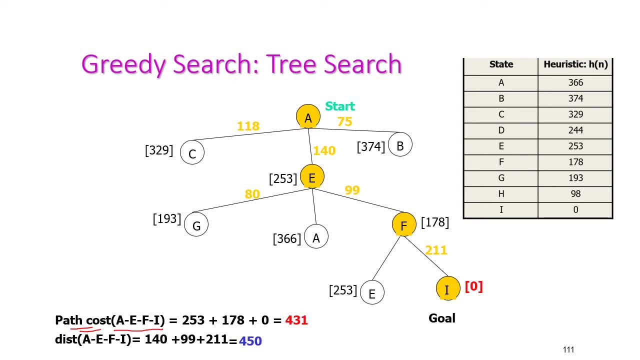 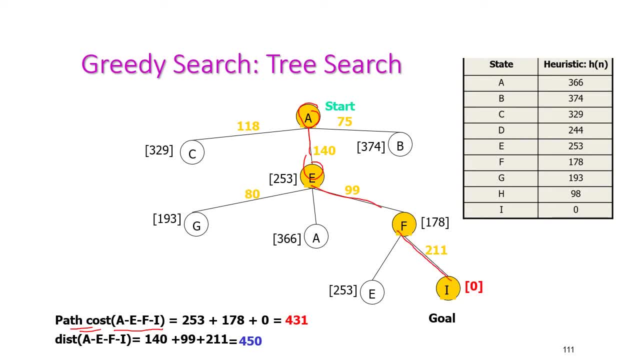 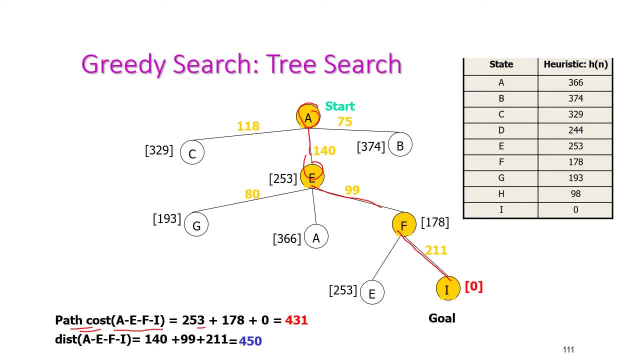 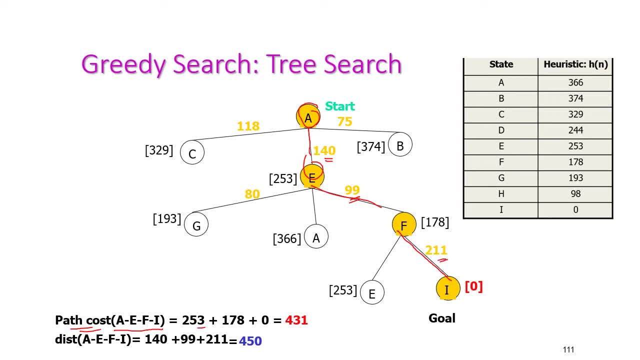 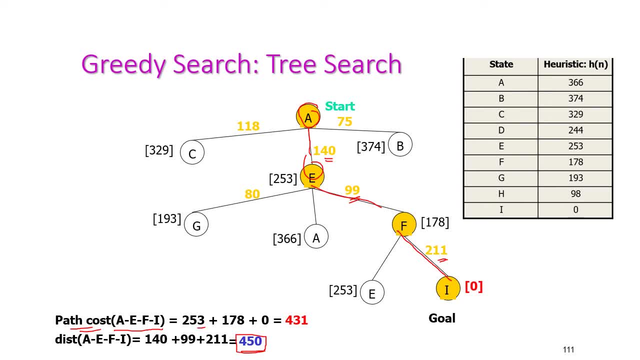 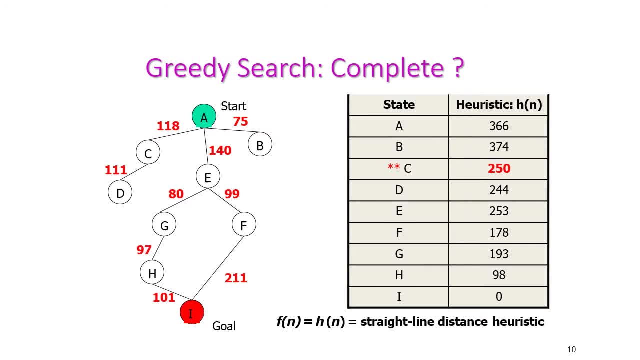 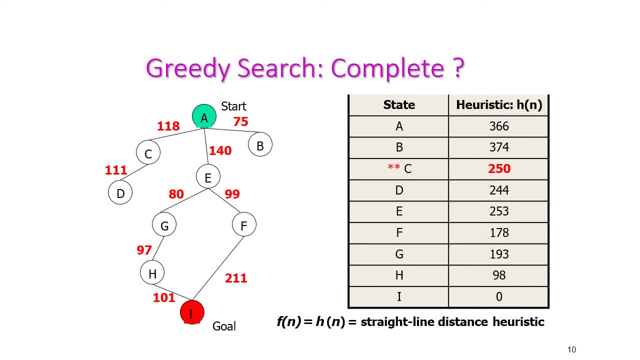 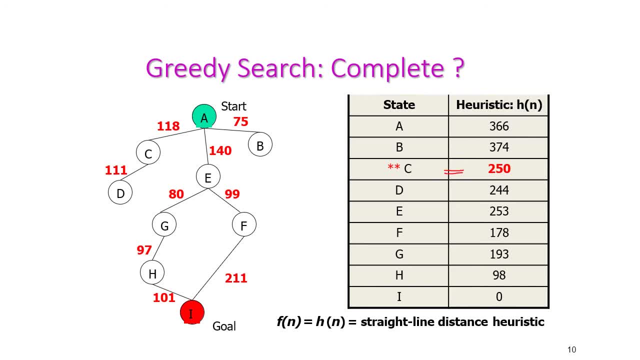 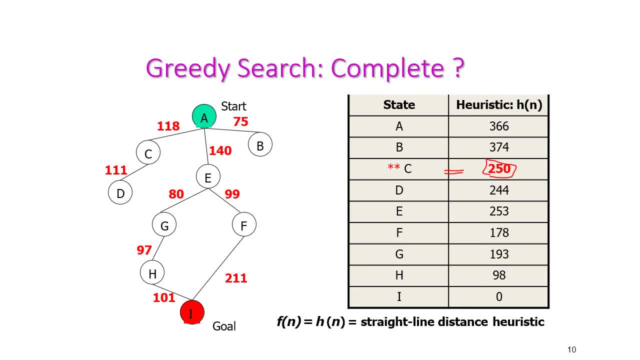 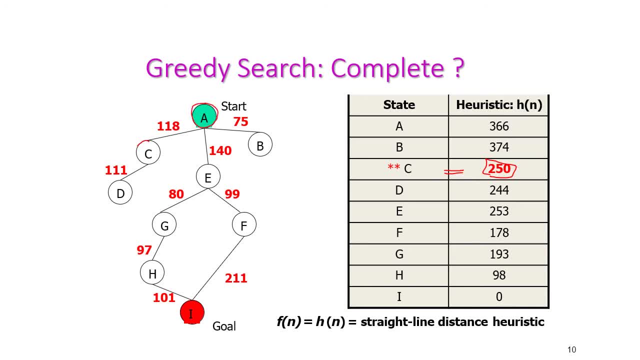 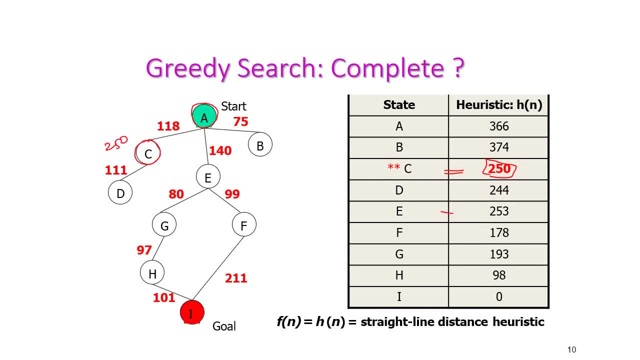 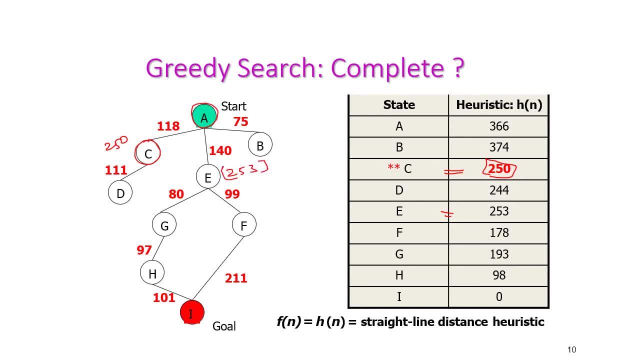 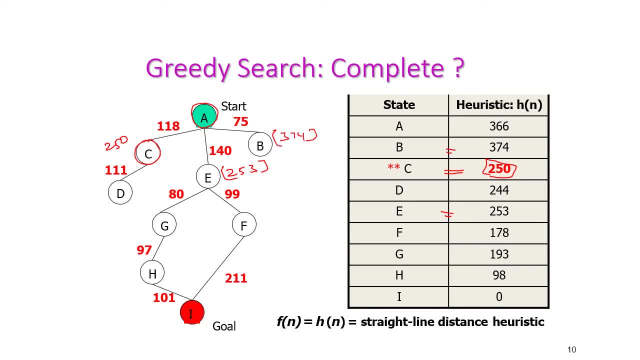 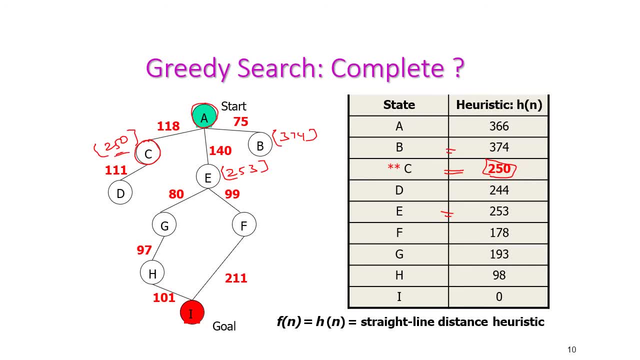 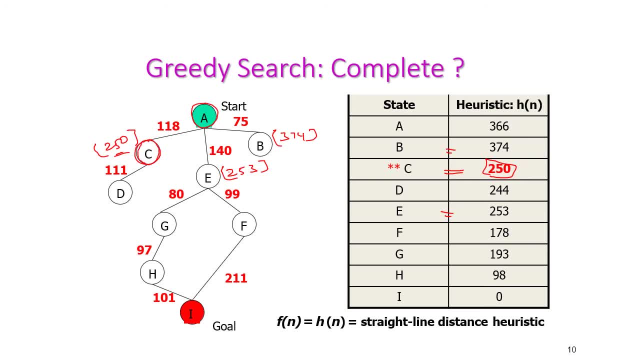 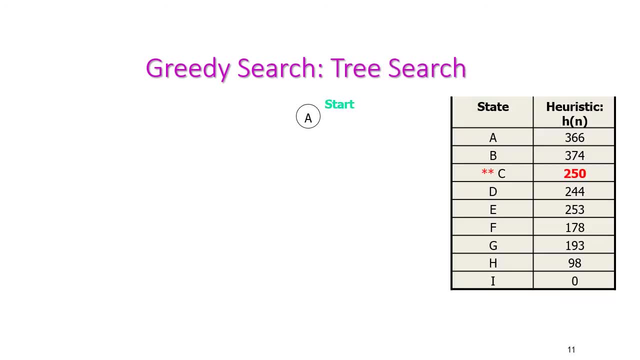 value. so we have to select only this c for further expansion. right, let us see what will happen in this situation. okay, so initially we can start from the starting state. is this heuristic value is 366. so from the starting state we are having three other states: c, e and b. the heuristic value of c. 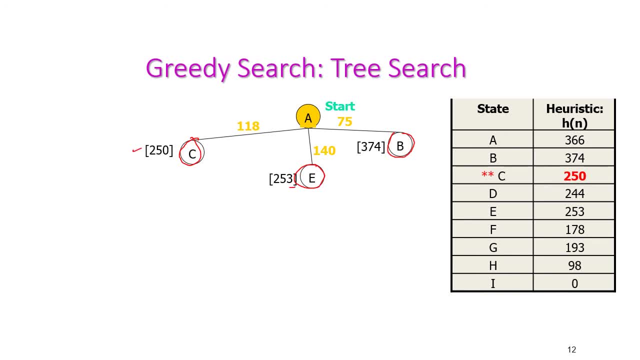 is 250. this is very much less when compared to the other two states. so we have select this. c is for further expansion. okay, from c. we are having the node d and a. okay, a is already visited, so we cannot go to a. okay, so d is the only option for us to expand further. from d we cannot. 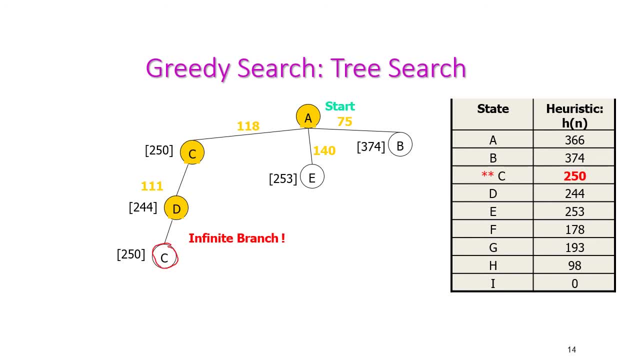 go back because c is already being visited, isn't it? so d, c, d, that will go on like that, okay, so we met the infinitive branch. infinitive loop will be there. okay, we cannot reach the gold state, so this is the one of the drawback when using the heuristic searching value. 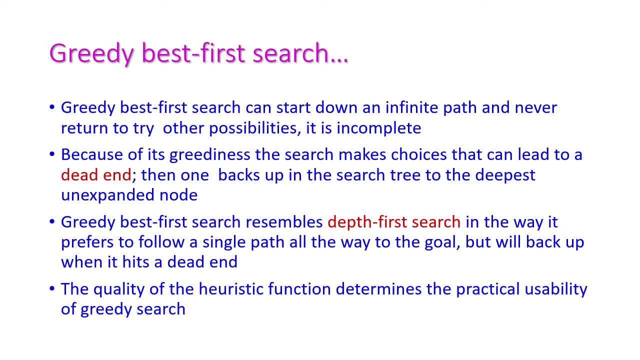 and the greedy best first to search can start down an infinite path and never return to try other possibilities. okay, so it is called as incomplete. okay, in our example, it it cannot restart our path, new search. okay, it cannot go back to starting state and it will not do the research for finding the root path. so this is the 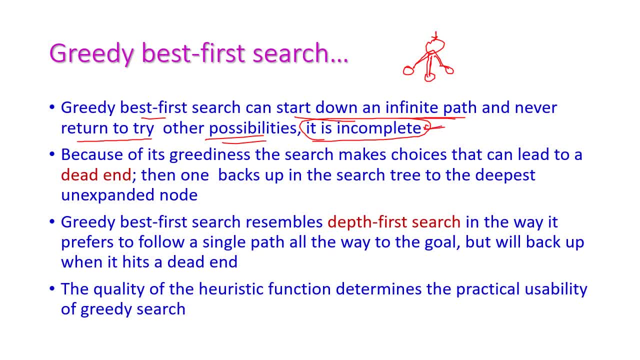 very big drawback of greedy best first search, and it because it will meet the dead end. and greedy best first search resembles depth first search in the way it prefers to follow a single path all the way to reach the goal- okay, but in the best first search it will go back up and hit the dead end. the quality of heuristic function.